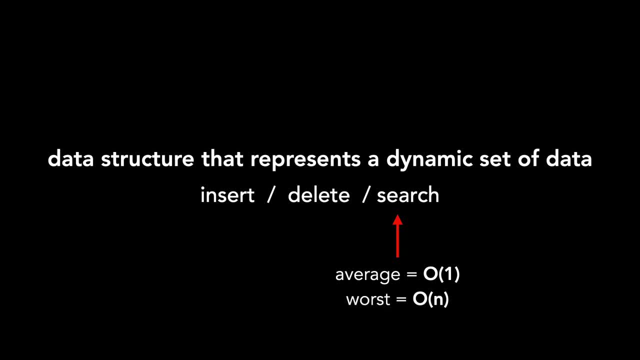 although this degrades to O in the worst case. I'll start by noting that the term hash table is sometimes used interchangeably with dictionary. Dictionaries represent a generic way to map keys to values. Hash tables are a specific way to implement a dictionary using 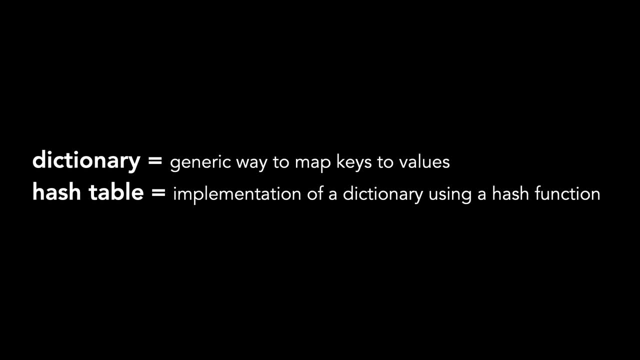 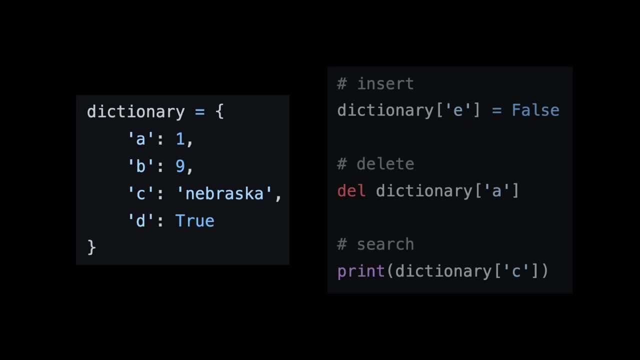 a hashing function. You've probably seen or worked with dictionaries or hash tables. if you've done basic programming, Here's Python code showing dictionary usage. Let's talk about our key function, hash table. To do this, we'll start by exploring a similar concept to hash tables called direct access. 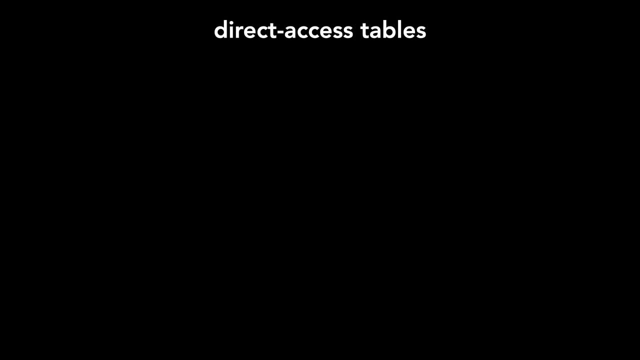 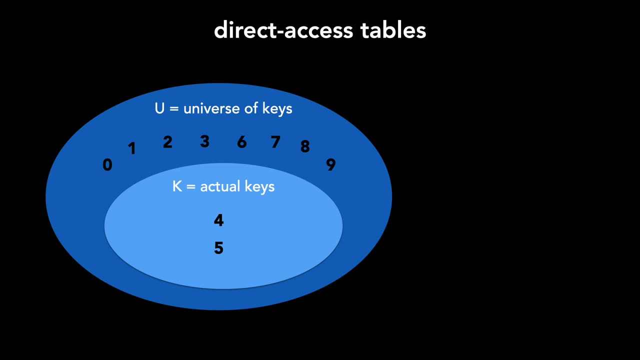 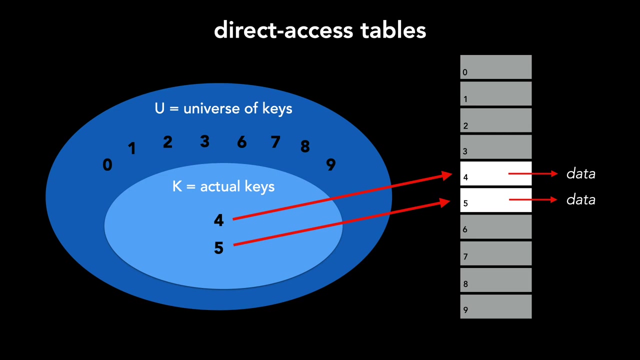 tables With direct access tables we have a universe of keys shown on the left. Some of the keys are in use and they point to data With direct access tables. insert, delete and search are all constant time operations. The key function hash table is used interchangeably. 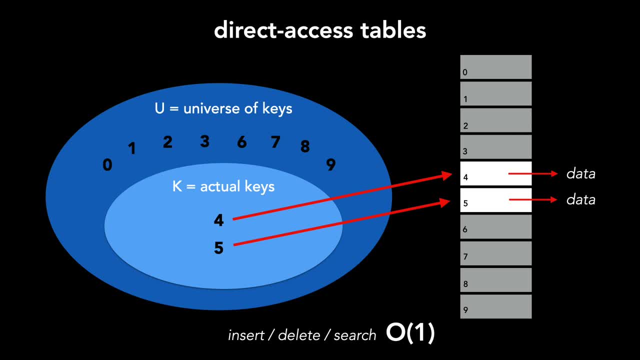 with constant time operations. In other words, a direct access table is an array And if you need to represent every key in the universe, we say: U is unbounded and impractical to store in memory. Enter hash tables. With hash tables, the space requirement is O, where k is the 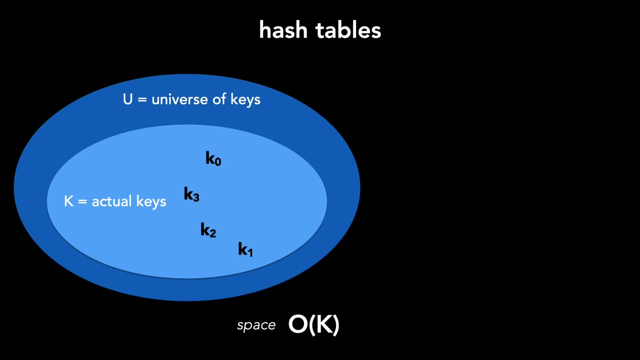 number of keys. To achieve this, we introduce a hash function. To do this, we insert a hash function and just hold k at the end. This is a simple hash function that maps keys to a location in the table that holds data. 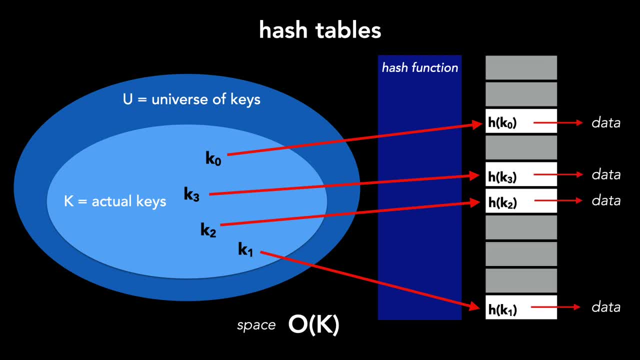 Because our universe of keys is no longer unbounded, it is possible that hashing two different keys may result in the same value, called a collision. One method to accommodate collisions is called chaining. To support chaining, we can use a method of appending two keys to a single object. 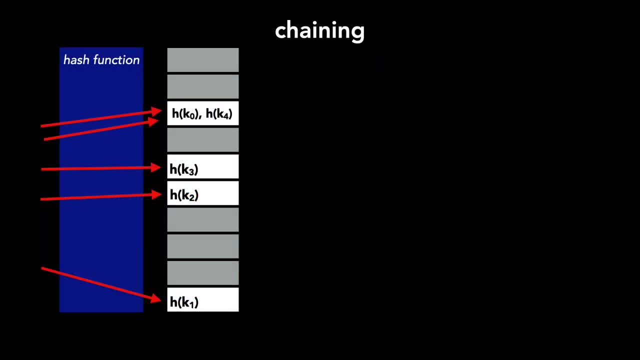 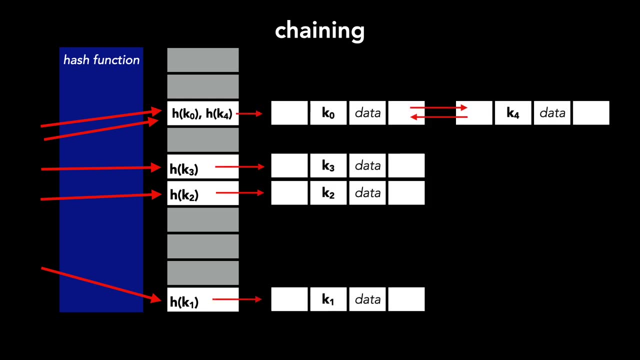 The first method is called chain. The second method is called chain. To support chaining, we introduce linked lists and our table locations become a bucket of values. To keep search as close as possible to O, we need a hash function that maximizes